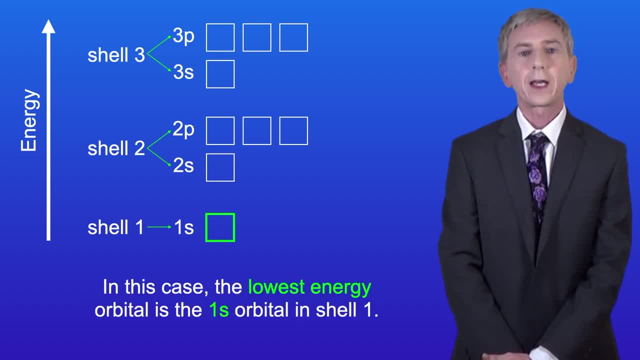 We're going to start with hydrogen, which has got one electron. In this case, the lowest energy orbital is the 1s orbital in shell 1.. So here's our electron, and you'll notice that we're using an arrow to show the electron spin. 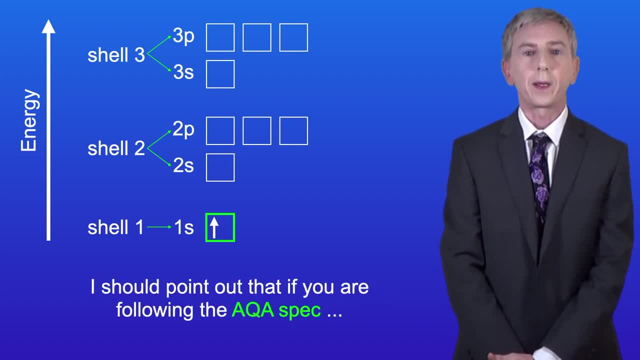 Now I should point out that if you're following the AQA spec, then you need to show an electron using an arrow like this instead. However, for the OCR spec, we show electrons using a normal arrow, which is what I will use Now. another way of writing this is to use a shorthand version showing just the subshells. 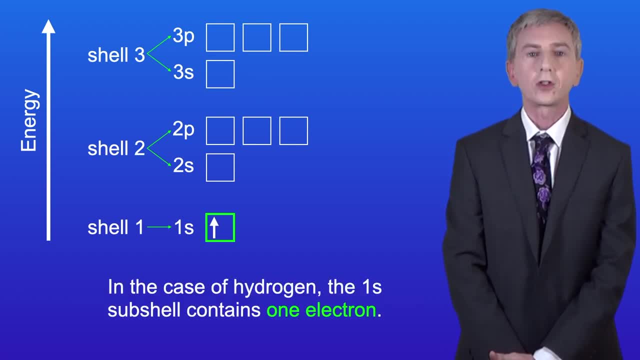 This is called the electron configuration. In the case of hydrogen, the 1s subshell contains one electron, So the electron configuration of hydrogen is 1s1.. Let's look at the element helium. Helium has two electrons. Again. the lowest energy orbital is 1s, so our first electron goes there. 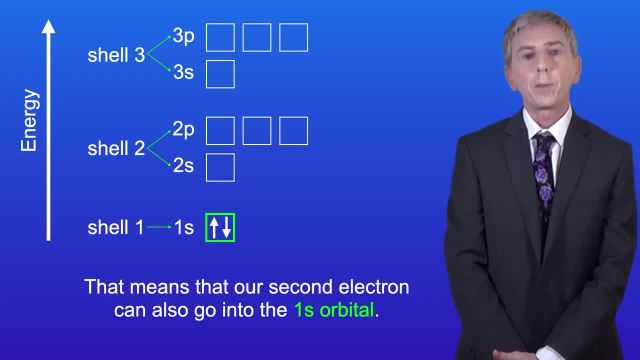 Remember that each orbital can hold up to two electrons, so that means that our second electron can also go into the 1s orbital. Now you'll notice that we flipped the spin of the second electron, and that's because electrons in the same orbital must have opposite spins. 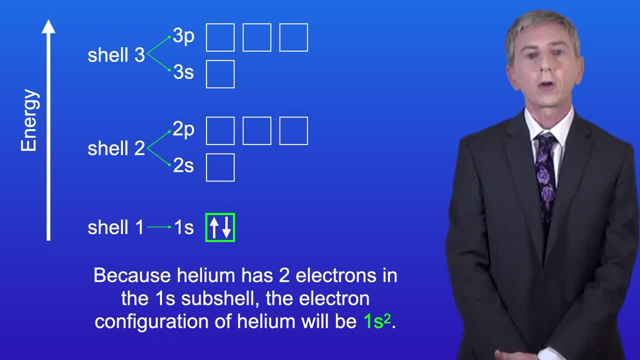 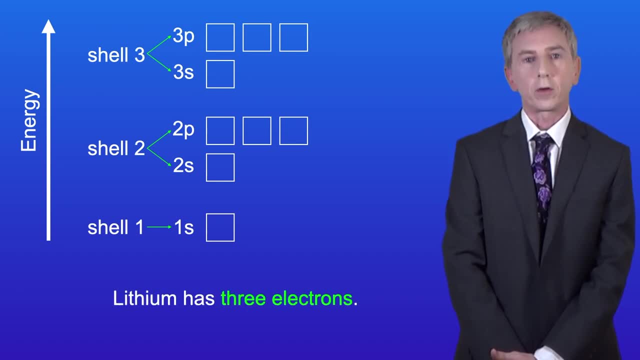 Because helium has two electrons in the 1s subshell, the electron configuration of helium will be 1s2.. Okay, let's look at lithium now. Lithium has three electrons. Again, we can put the first two electrons into the 1s orbital like this: 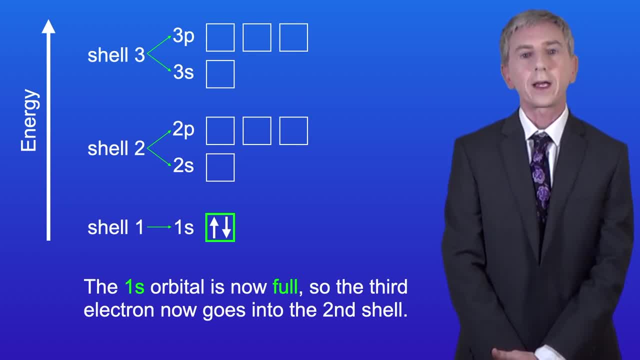 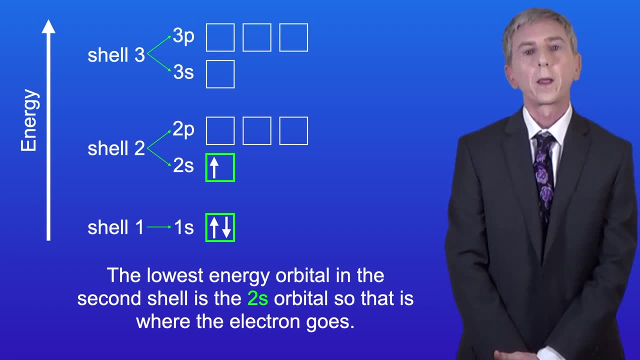 The 1s orbital is now full, so the third electron now goes into the second shell. The lowest energy orbital in the second shell is the 2s orbital, so that's where the electron goes. This means that the electron configuration of lithium is 1s2- 2s1.. 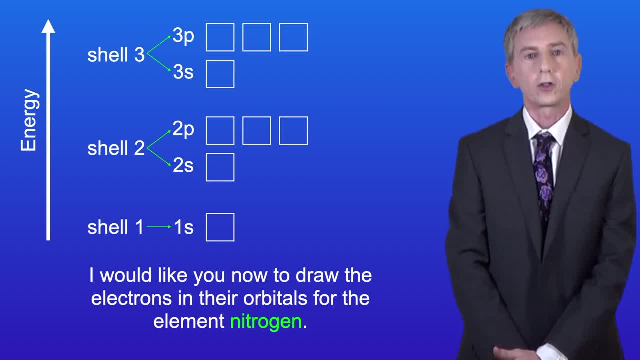 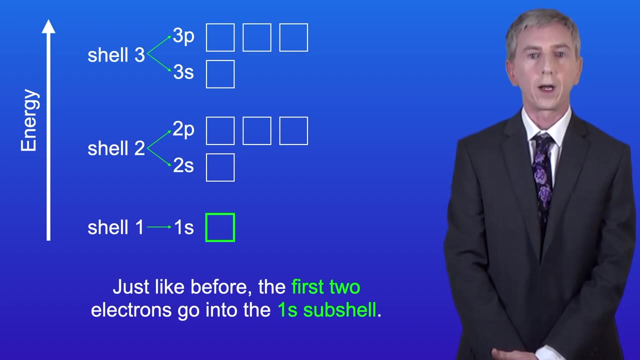 Okay, I'd like you now to draw the electrons in their orbitals for the element nitrogen. Nitrogen has got seven electrons. I'd just like you to work out the electron configuration for nitrogen. so pause the video and try this yourself. Okay, so, just like before, the first two electrons go into the 1s subshell, and here they are. 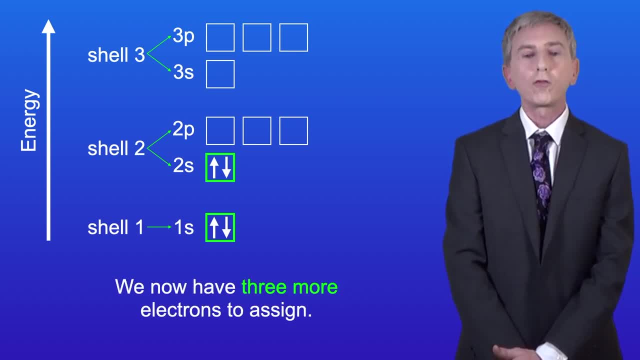 The next two electrons go into the 2s subshell. We now have three more electrons to assign. Now you'll notice that all of the p orbitals in the 2p subshell have the same energy. Remember that if we've got orbitals with the same energy, then we put electrons into individual orbitals before we pair them.